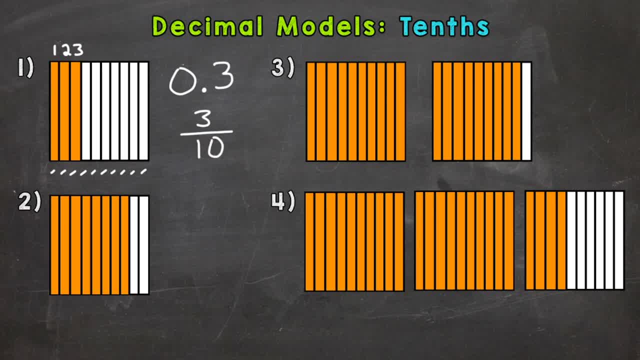 Three tenths, Three out of ten. That decimal and the fraction both have the same name: Three tenths. They just look a little different. One's a decimal, One's a fraction. So let's go on to number two, And again we're working with tenths, So it's cut into 10 equal pieces, And each one of 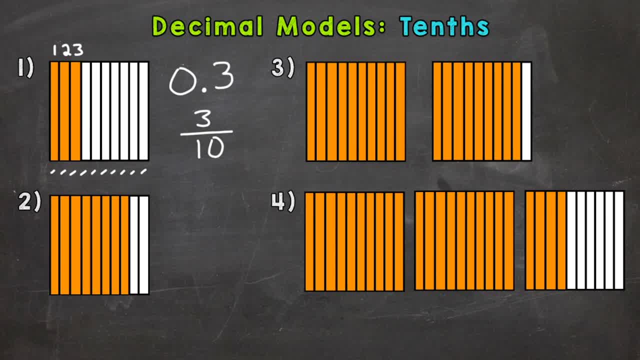 those pieces is worth one tenth. So let's see how many we have filled in. We have one, two, three, four, five, six, seven, eight. So that model represents eight tenths or eight out of ten. So there's the decimal, and then 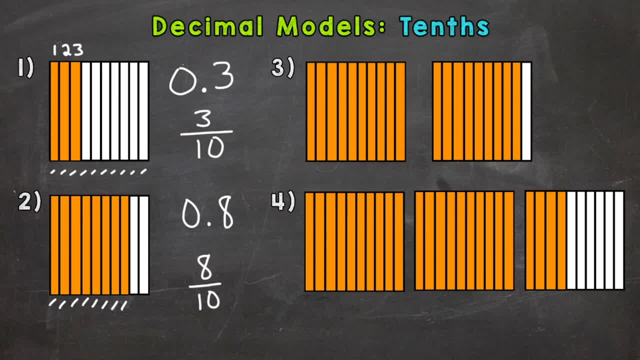 here's the fraction, So eight tenths is just under one whole. We almost have that full square filled in, but not quite, So we're not quite up to one whole. So let's move on to numbers three and four here, where we're going to have a whole number with a decimal, So for example number three. 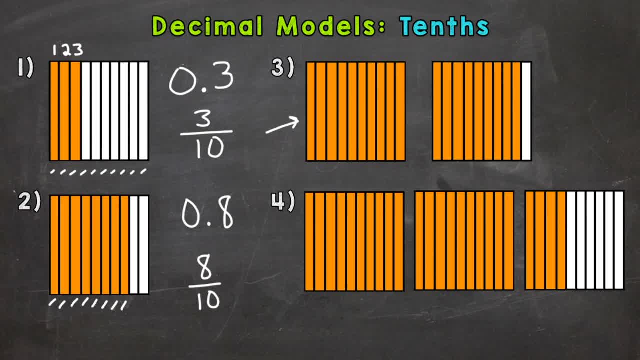 four, five, seven, eight. So if we have a two third 거죠 in and we have a decimal number- eight and then six, we're going to have a whole number with a decimal, So one besides five, and 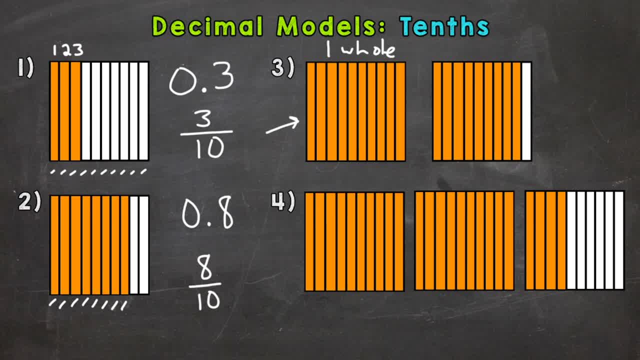 six. so we've got a whole number with a decimal number. That is what we're going to. we're going to look into next on our project, so long as it's full. So let's go ahead and develop our problem here. So remember, we want to graph one square as a whole. Now, the first one we want to. 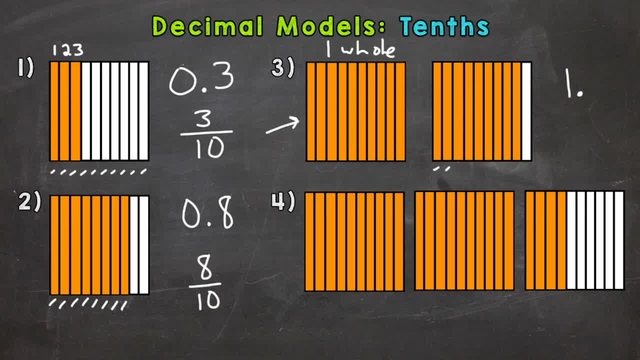 do. let's say, we're doing our first square, So we're going to be doing here is we're going to ад four, five, six, seven, eight, nine, So that second square represents nine-tenths, So we have one whole. 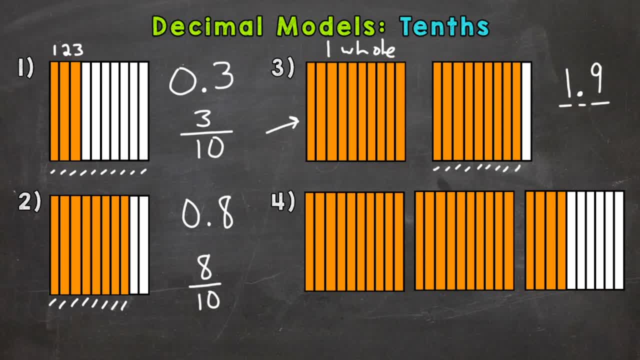 and nine-tenths, Or we can write it with a fraction, which means whole number and a fraction here one and nine-tenths And lastly number four. it looks like we have one whole, two holes, and then one, two, three, four-tenths. So we would have two wholes and four-tenths, Or 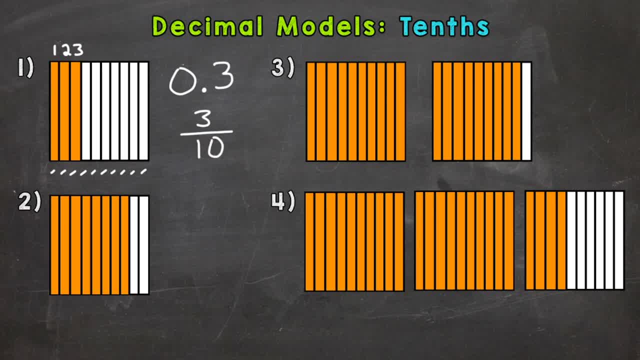 Three tenths, Three out of ten. That decimal and the fraction both have the same name: Three tenths. They just look a little different. One's a decimal, One's a fraction. So let's go on to number two, And again we're working with tenths, So it's cut into 10 equal pieces, And each one of 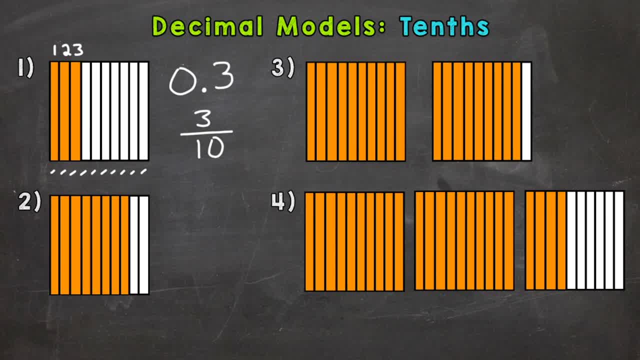 those pieces is worth one tenth. So let's see how many we have filled in. We have one, two, three, four, five, six, seven, eight. So that model represents eight tenths or eight out of ten. So there's the decimal, and then 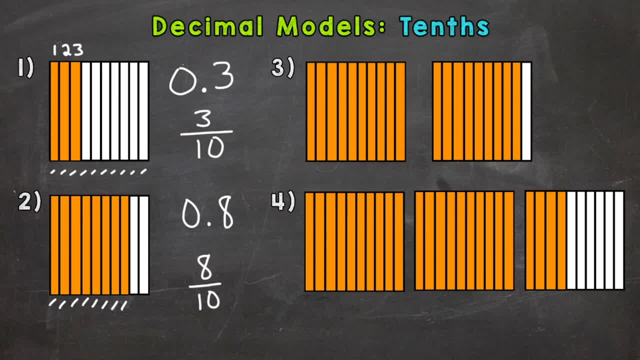 here's the fraction, So eight tenths is just under one whole. We almost have that full square filled in, but not quite, So we're not quite up to one whole. So let's move on to numbers three and four here, where we're going to have a whole number with a decimal, So for example number three. 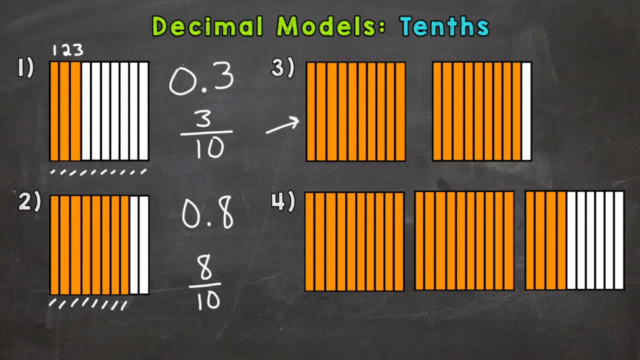 four, five, six, seven, eight. So we have a whole number with a decimal. So that represents one whole. Now the second square is almost filled in, but not quite. So it's almost a whole, but not quite there. So we're going to have a whole and then a decimal. So let's put one whole decimal. 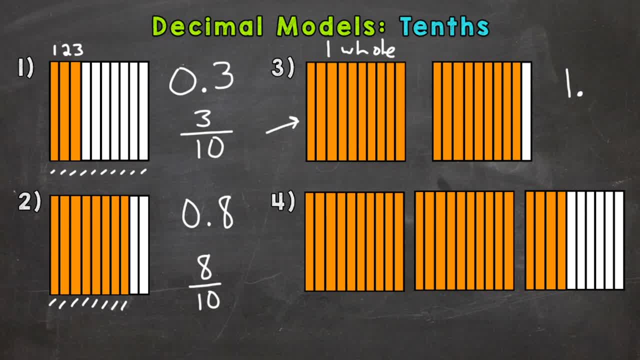 and let's see how many tenths we have filled in for that second square: One, two, three, four, five, six, seven, eight, nine. So that second square represents nine tenths. So we have one whole and nine tenths, Or we can write it with a fraction, which means whole number and a. 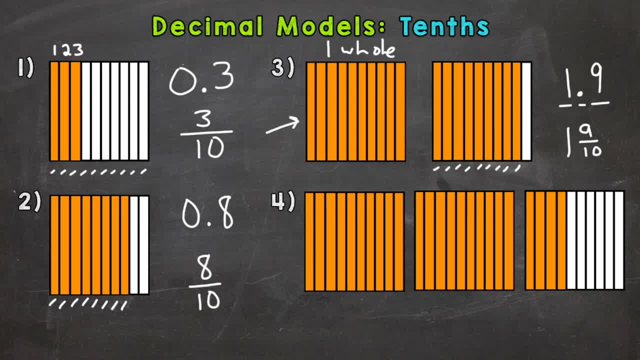 fraction here, one and nine tenths And lastly number four. it looks like we have one whole, two wholes and then one whole. So we have one whole, two wholes and then one whole, two wholes, One, two, three, four tenths. So we would have two wholes and four tenths, Or two and four tenths.